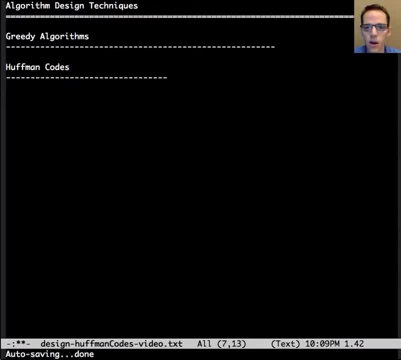 This is Dr Carol, and this video is about Huffman Codes. Huffman Codes are a great example of greedy algorithms. The point of Huffman Codes is to achieve file compression. The ASCII code has approximately 100 printable characters and a handful of non-printable characters. Each character requires 7 bits of information because that is a log base. 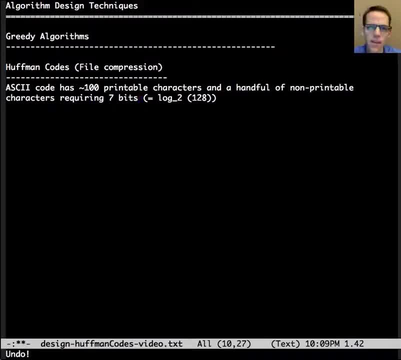 of 128.. Then there is an eighth bit for parity. It takes one byte to store an ASCII character. For example, the ASCII character value 7 is a beep. That is an example of a non-printable character. Try printing it sometime. Tick backslash, beep untick. 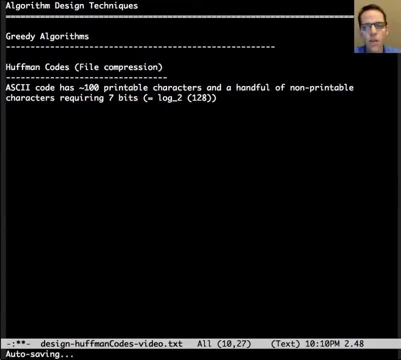 The way Huffman Codes work is to assign the frequent characters, the shortest codes, and you can reduce the number of bits required and hence the file compression. This can generally save about 25% of storage space for large files and 50-60% for some large. 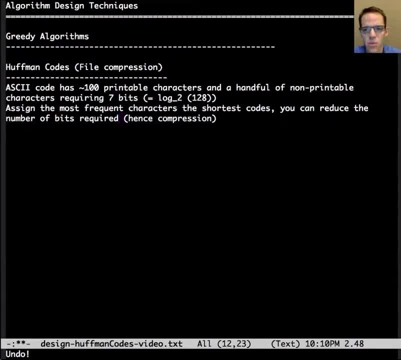 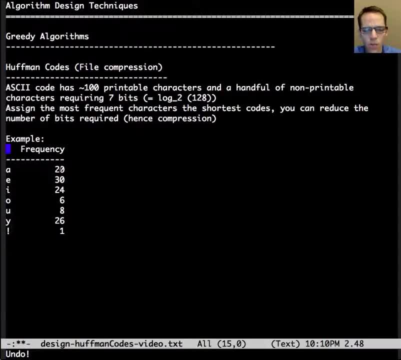 E A O U Y exclamation mark. Why not include these when we have the following frequencies: These are the license names which will appear only when it happiness lists are specified here, Then, because we only have your number here, we can encode them with just 3 bits In the 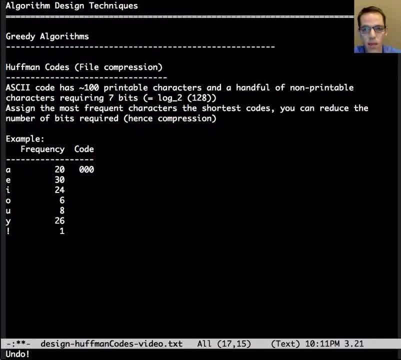 configuration table numbers. order for each number sounds스, and we can encode the machine of them faithfully. Now, if we did this, we'd have the following total bits- and this is just the frequency times by the number of bits here. So for A we'd have: 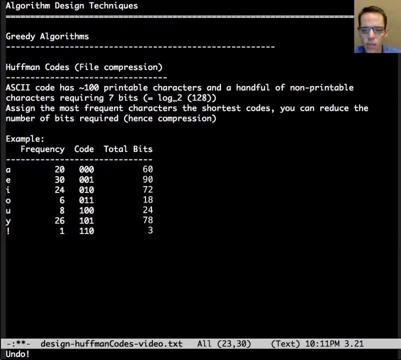 60,. for E we'd have 90. And so what we'd really like to do is reduce the ones that have a higher frequency. If we can give them a smaller code, that will reduce the total number of bits needed to store it. So here in this example, 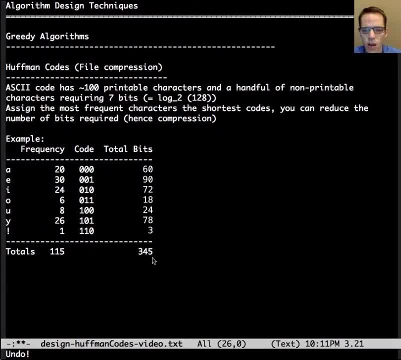 we have 115 characters in in this file and therefore requiring 345 bits. Now, characters with Huffman codes are only going to be stored at the leaves, only at the leaves of this tree that we're going to build And when we traverse the tree, 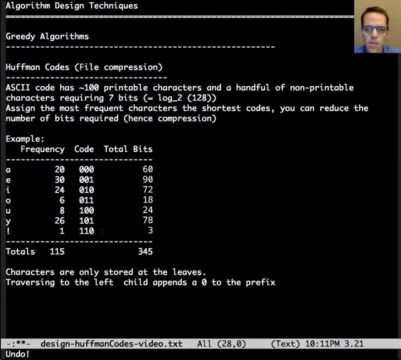 if we traverse it to the left, we're going to append a zero prefix to that letter. When we traverse it to the right, we're going to append a one letter to the prefix. So let's see an example that illustrates. let's see the tree that. 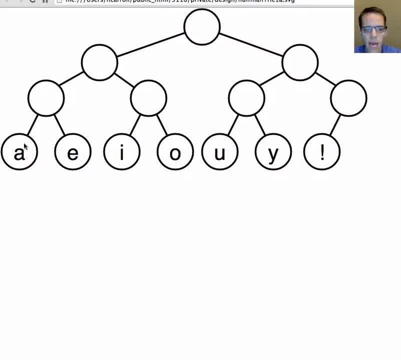 illustrates this example. Here we have it: A, E, I, O U Y, an exclamation mark. Now, as I mentioned, if you traverse left you, you append a zero to the code left, left. So, as I mentioned, A is zero, zero, zero and E is one, zero, zero, one, and so on, And that's. 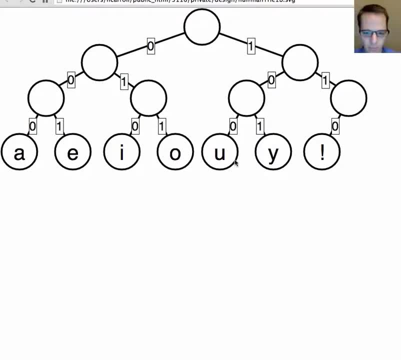 how we get the code, each of these letters, in the Huffman codes for it. Now we can improve a little bit upon this. and then you notice there's no child, there's no right child here. So if we have a 1- 1, we already. 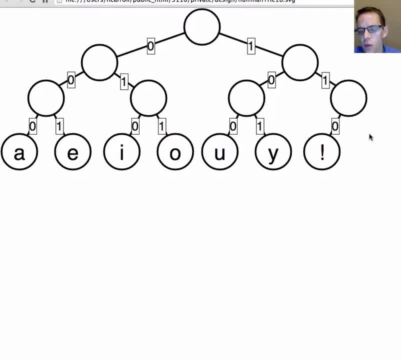 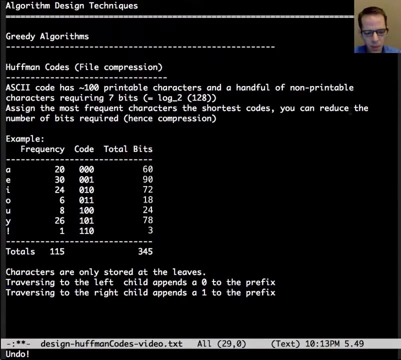 know that it's going to be an exclamation mark because there's no right child, So what we could do is just actually move this one up, which is going to reduce the number of bits needed. In this case not very much, because the exclamation mark was infrequent. And so then, if we had the 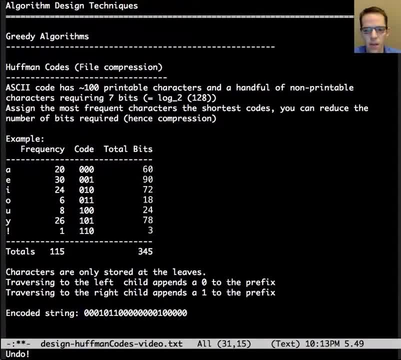 encoded string 0, 0, 0, 1, 0, 0, etc. that would be decoded into A, because we would notice we'd just follow pattern 0 0, 0.. Okay, well, that has to be A, And then the next one. well, one doesn't uniquely. 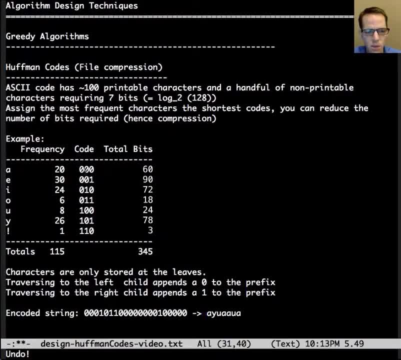 define anything. So 1 0, that doesn't uniquely define anything. So 1 0 1, 1 0 1, that's Y. We start over. well, 1 doesn't uniquely define anything. So 1 0,, no, 1 0 0.. And then we have U, And then we have 0 0 0 A, 0 0 0 A. 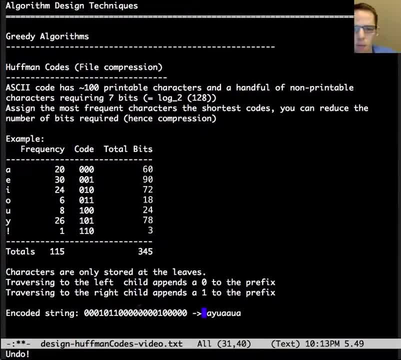 And then we get U and A. So that's how this is encoded, But we haven't saved anything yet. So this is this is the normal case that we're trying to beat. This is, this is pretty much how your your. 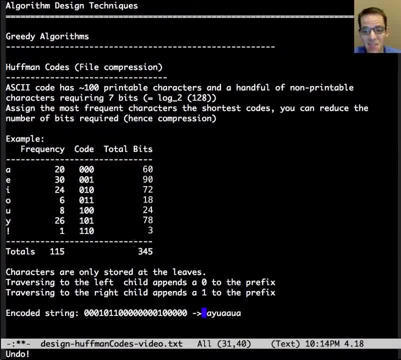 well, like this video text file actually is stored, something very analogous to this. It's all stored and we know exactly how to read it. Okay, But so now what we're trying to do is we're trying to compress the file and save some bits. So Huffman, a couple of years ago, presented the 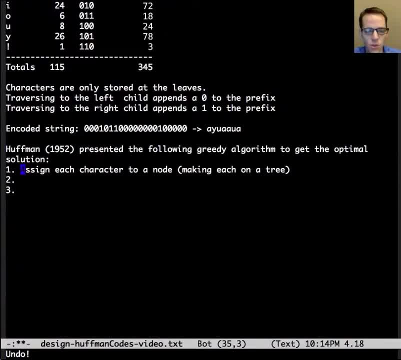 following greedy algorithm to get the optimal solution: First, assign each character to a node and thereby making it a tree, Okay. And then we'll assign the frequency of that character as a weight, And we're going to work with the trees based on their weights. 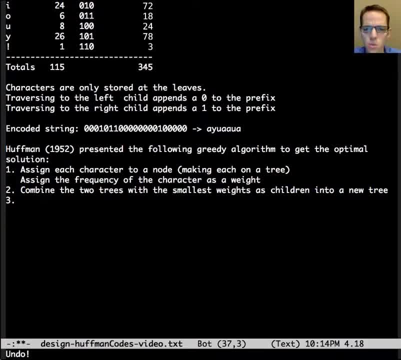 Step two, then, is to combine two trees with the smallest weights as children into a new tree and assign the weight of the sum of the children as the weight of its tree, And you probably guessed it. Step three is repeat step two until all the trees are combined. 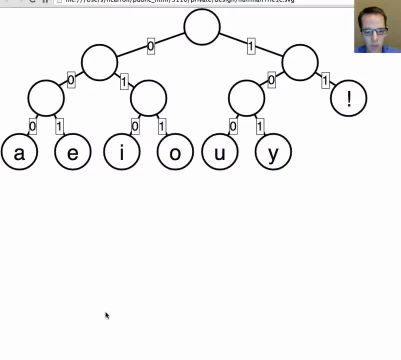 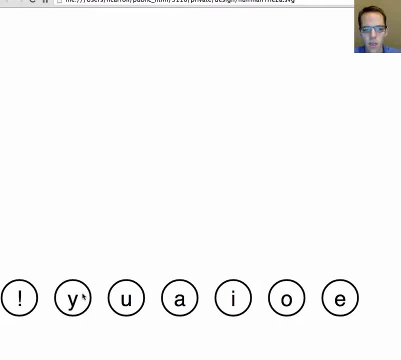 Okay, Well, let's see an example. So here we have the same set of letters, except I've sorted them so that they're in the order of least frequent, because that's how we're going to combine them. So step one was make all the nodes and assign weights. Check, We're done, Okay. Now step two was combine the smallest two trees. 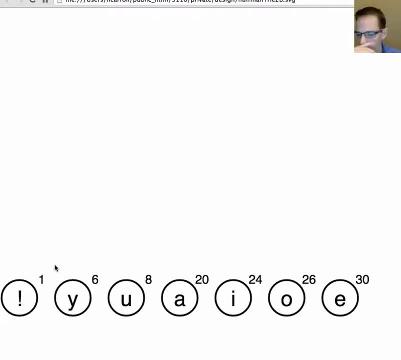 in into children of a new tree. Okay, Well, that's going to be these two, and all of these are trees, and so, and we'll label the new tree t1, and then we've updated its height to be 7, because there's 1 plus 6, and this, these numbers. 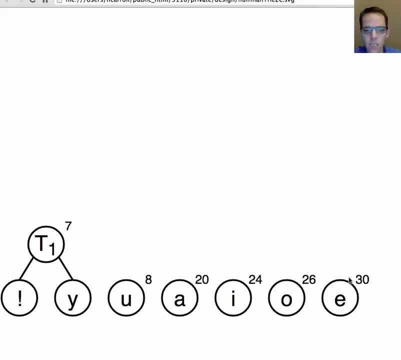 remember, are the frequency of the letters. so e is the most frequent and so we want to have the shortest code for it. and then step 3 was repeat. okay, let's see the smallest two sub trees. smallest- sorry, smallest- two trees that'd be. this one was 7 and this one with 8. we combine them, update it to 15. smallest 2: 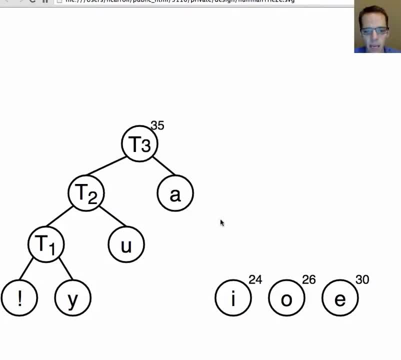 is going to be 15 and 20, okay. smallest 2: oh, it's 24 and 26 here, so we'll combine them to get 50 here. now, smallest 2 would be 30 and 35, so we'll combine them, then we'll smallest 2 and then we're done. we've combined them all now to get the. 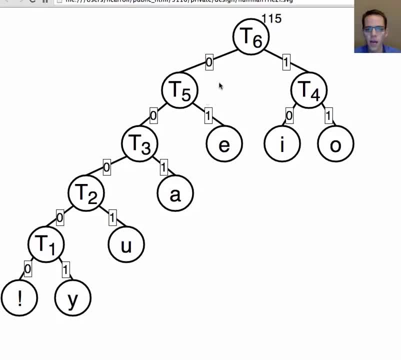 Huffman codes. all we need to do again is apply the 0 for the left child and the right for the, the, the one for the right child, and then, if we follow this for example exclamation mark, we, we determine 0, 0, 0, 0, 0, and then Y would be 0, 0, 0, 0, 1 and all. 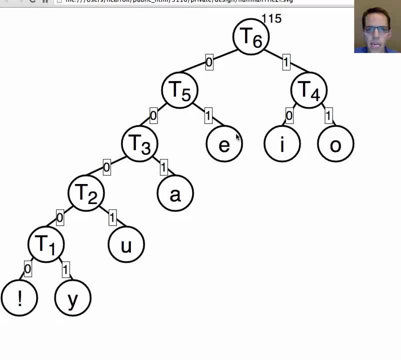 the letters accordingly. so notice that e has a very short code- 0, 1- and it's the most frequent, and so we want to have the shortest code for it. and then step 3 was the least frequent, so we've reduced the amount of code needed for here by one. 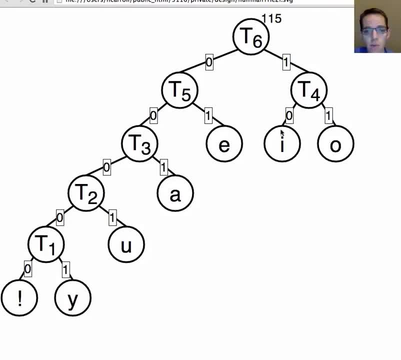 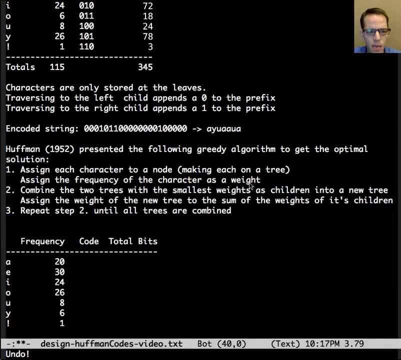 but it was the most frequent, so that was a big gain. we've also reduced it for, I know, at the same time, so that that was a big game. let's see how that works out. okay, we build this table again with our frequencies or letters and their codes, so then we have one, if we're starting. 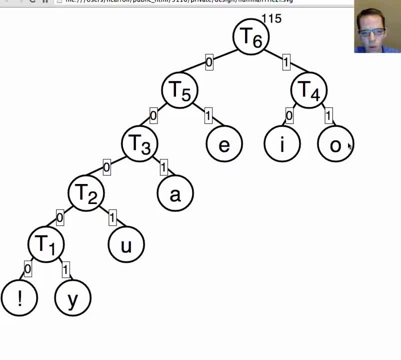 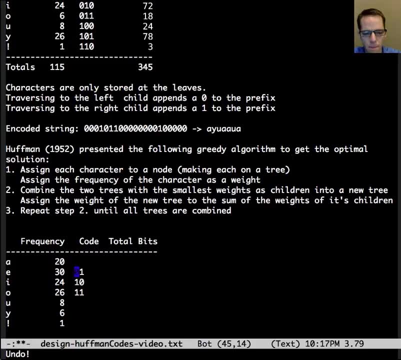 from the right. we're gonna- oh was one, one, seven, so we're gonna go off this table 0, and then we're done with by one. So this is how we make the MYA stands: here was 1, 1 is its code, and I is 1: 0, and then e is 0, 1, 0, 1, and then 0, 0, 1, 0, 0, 0, 1.